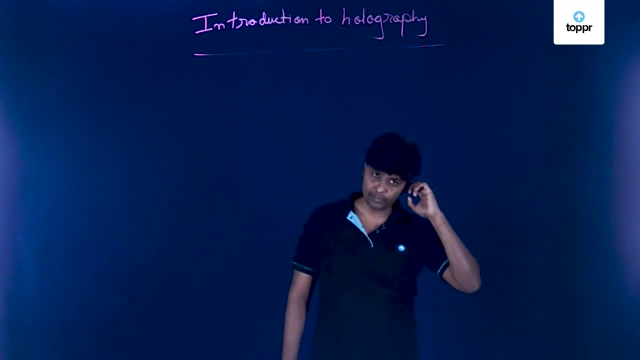 negatives. Using these negatives you can develop more photographs, right? If you? if you ask your father or if you ask your parent, they will tell you about this. So negative is the inverse of the photograph. That means, if you see the negative carefully, something. 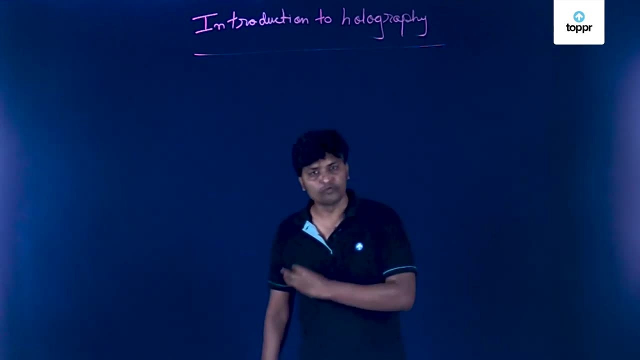 which is very bright in the photograph will appear like this: This is the photograph. appear very dark in the negative. So that means it is completely inverse of the photograph. The negative is completely inverse of the photograph. So that means what does this camera do? 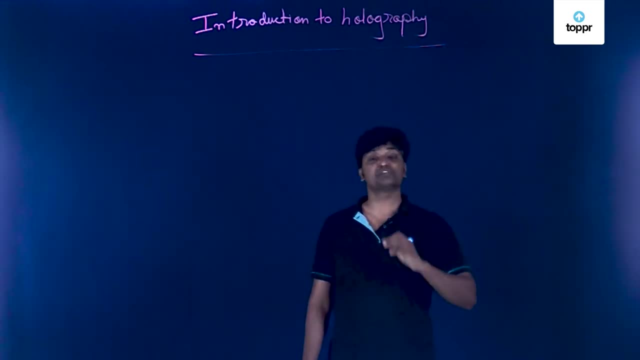 It captures the intensity of the light, intensity of the reflected light. If the intensity is less, then the negative will be very, very it will not be dark. If the intensity is more, the negative will be dark, So that when we develop it, we get exactly the opposite of this. 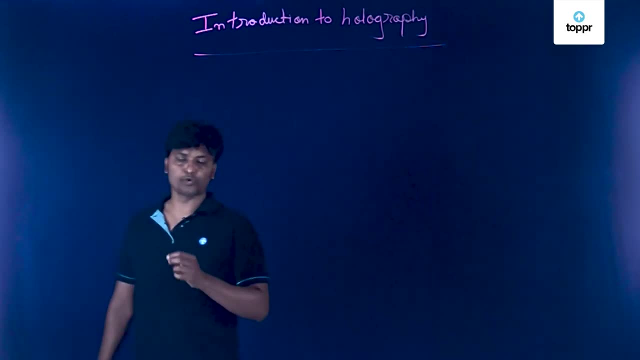 However, in holography, what we do is, along with the intensity of the light, we also capture the phase, the information of phase. We also record the information of phase. The moment we record the information of phase, what we do is we are actually recording the. 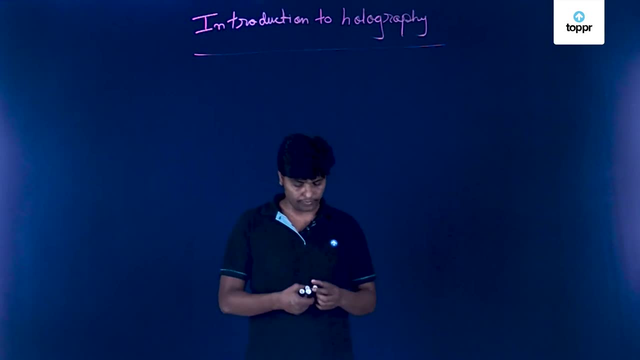 information of depth of the object. Right Now, let's say, for example, if you click a photograph of this particular pen, what will happen is you will see only the 2D image of the pen. Why? Because your photograph, Your camera, will capture the intensity of the light which is getting reflected and getting. 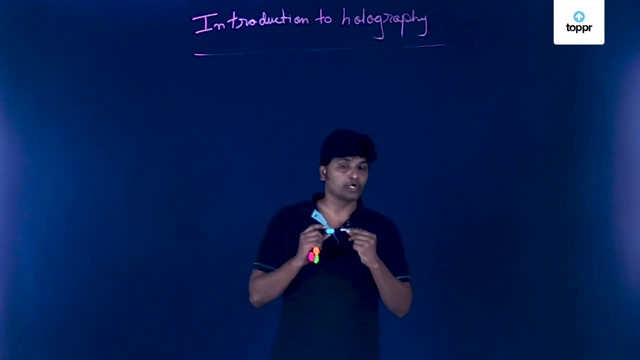 entered into the camera. However, in holography, you just not record the intensity, you also record the phase Right And, using the phenomenon of interference, you can create a 3D image of this pen, which is called as holography.